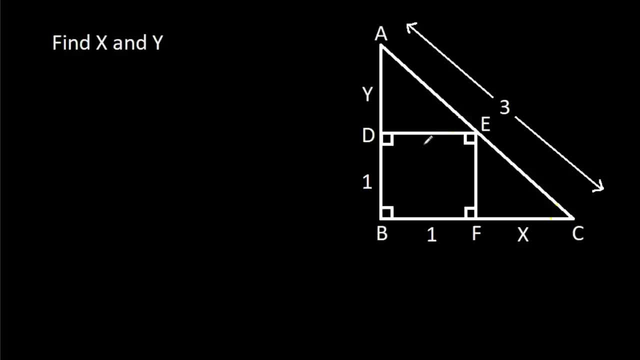 In this video we have been given a square inside a triangle: ABC and BD is 1,, DA is Y, BF is 1,, FC is X and AC is 3, then we have to find X and Y. So BDEF, it is a square. 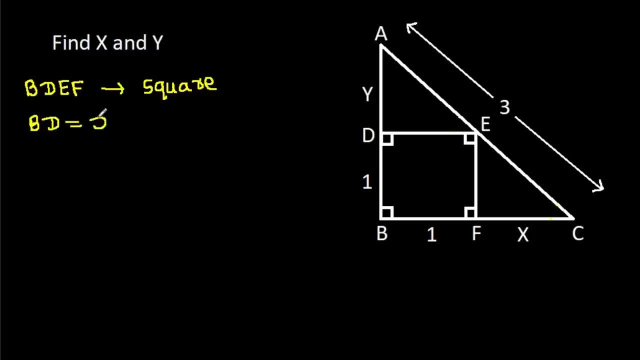 that means BD, it will be equal to DE, it will be equal to EF, it will be equal to FB. that will be 1.. So DE it is 1 and EF is 1. And BC it will be parallel to DE. that means these two angles, they will be equal. 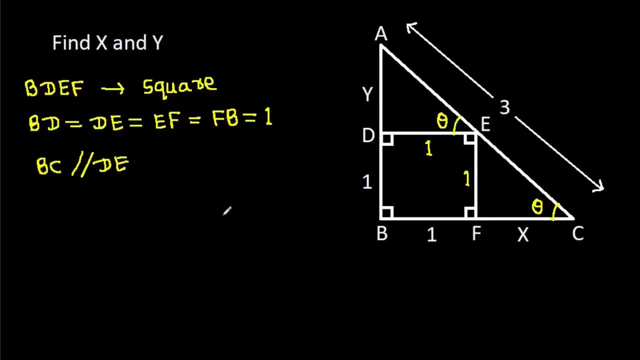 Suppose theta. and now inter angle ADE tan theta, it will be AD by DE, that will be Y by 1. And inter angle EFC tan theta, it will be EF by FC, that will be 1 by X. 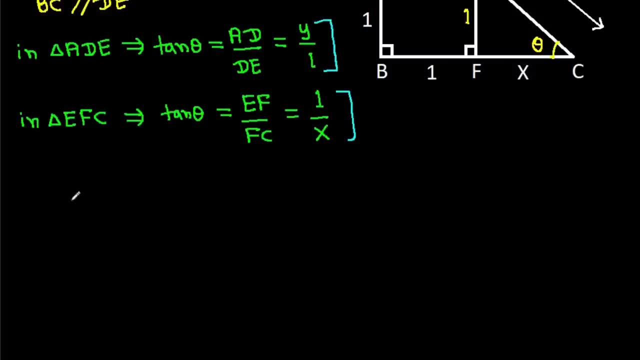 So from these two equations we can say that Y by 1, it will be equal to 1 by X. So we get Y is 1 by X. So if we get V, then V is 1 by 1, and we have to do V pressing 4 by 4,. 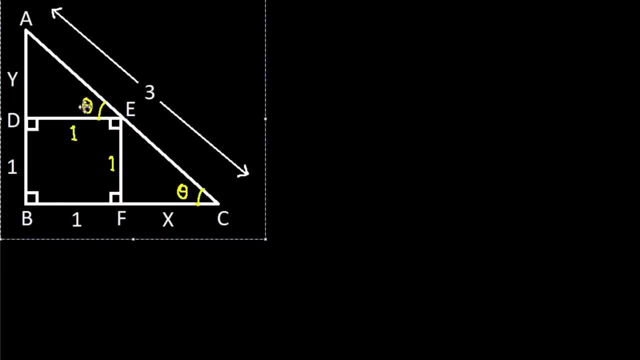 each of these angles. So one angle can beava when entry angle of 1 by 1, L by 1, and tác is where mentre angle is equal to one angle up. you take the angle up in the formula. So we do: EF is 1.. We are going to take a simplifying term to the square. 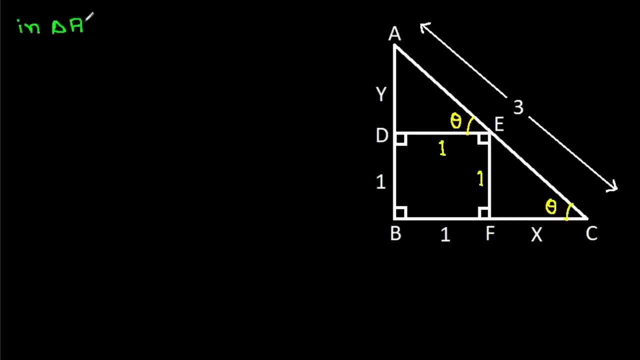 because this is the same as before minute. 않아 is equal to 1.. So by pulling out Horaren can we get that AMB, which is AB, over here. gera angle plus AMB over slippage plus BC square, it will be equal to AC square by Pythagoras theorem And AB it is. 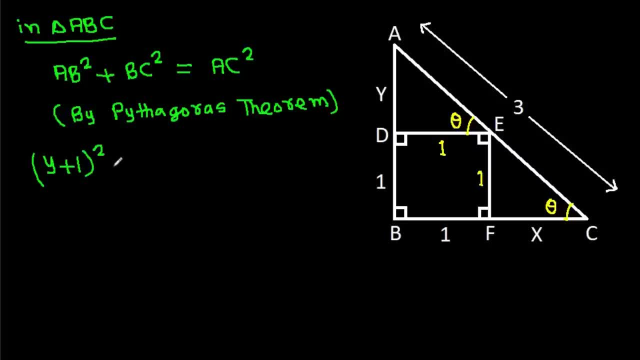 y plus 1 s square plus BC, it is 1 plus x square. it is equal to AC is 3 s square, and it is y square plus 1 plus 2y plus 1 plus x square plus 2x. So y square is equal to 9 and we have y is 1 by x. 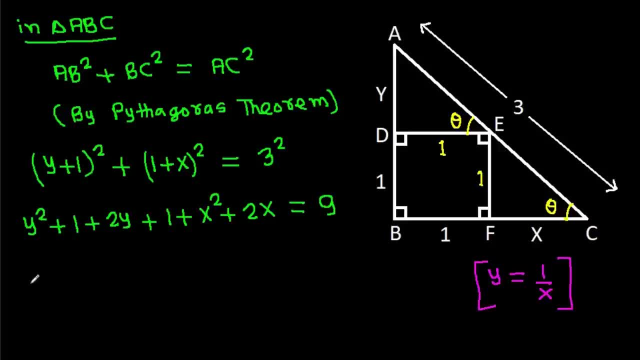 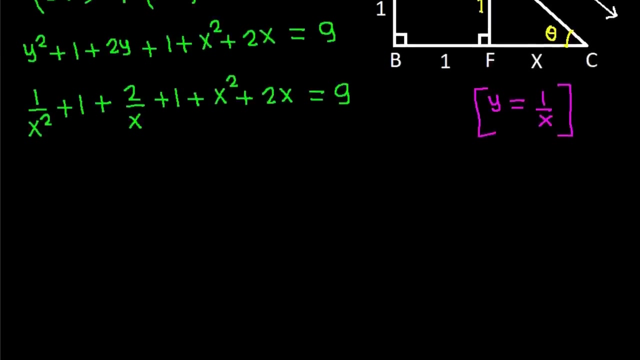 So y square, it will be 1 by x square plus 1 plus 2y, it will be 2 by x plus 1 plus x. square plus 2x, It is 9.. And it is x square plus 1 by x square plus, and 1 plus 1 will be 2 plus 2x plus 2 by x. 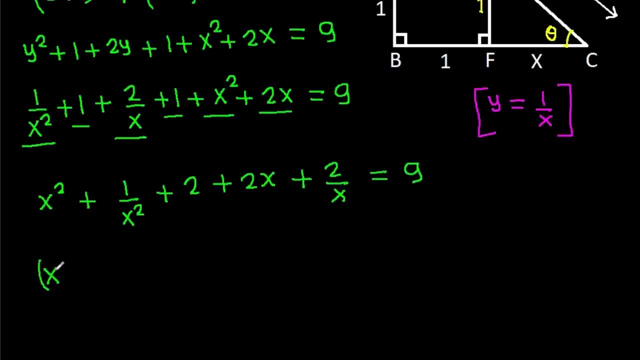 It will be 9.. And it is x square plus 1 by x square plus, and 2 is 2 times x, times 1 by x, minus 2x plus 2 by x, And then it is lowercase is equal to 9.. 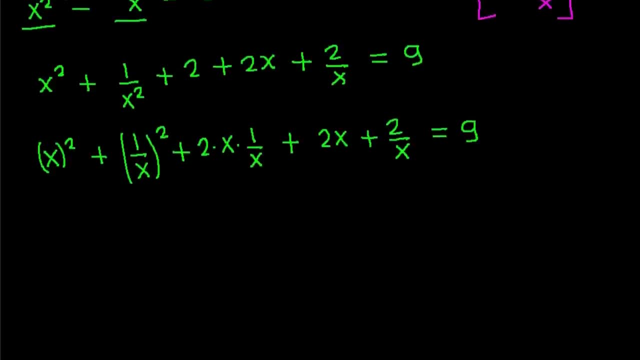 So we have given the number x, half by x, half minus 2 only, And then it is minus 1 by x, It is equal to 9. And then we have done thelied term From 4. From 4.. 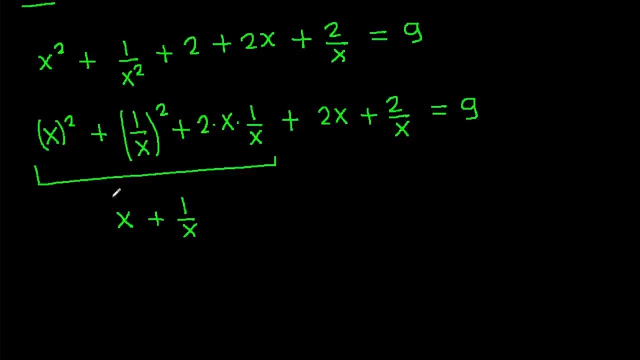 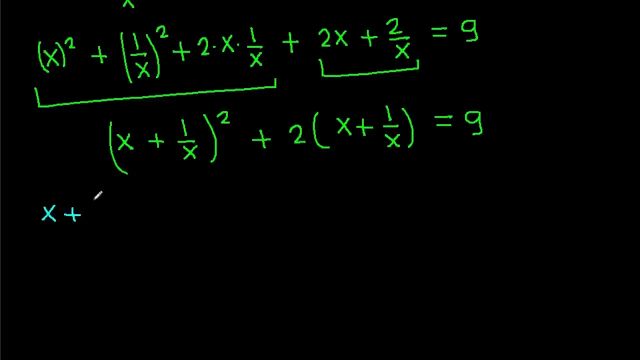 And the uses theWill come x plus 1 by x s square plus, and here we can take two common and it will be x plus 1 by x. that is equal to 9. and now, if we take x plus 1 by x is equal to t. 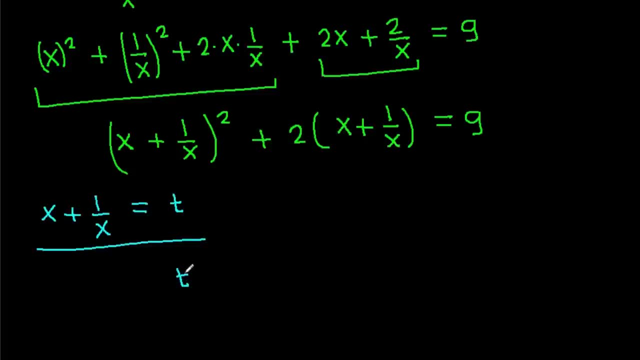 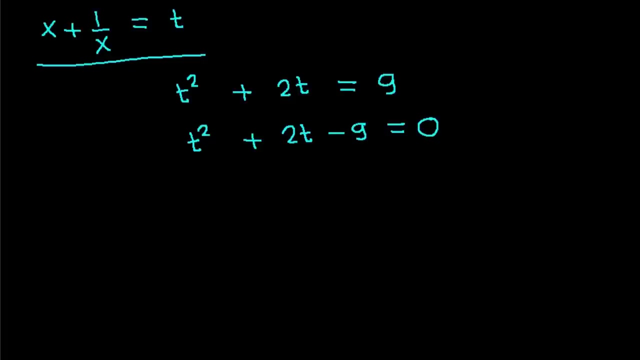 then it will be: t square plus 2t is equal to 9, and it is t square plus 2t minus nine is equal to zero. and now for equation AX, y square plus BX plus c is equal to 0,. x is equal to minus b plus minus s. square root of b square minus 4ac by 2a. 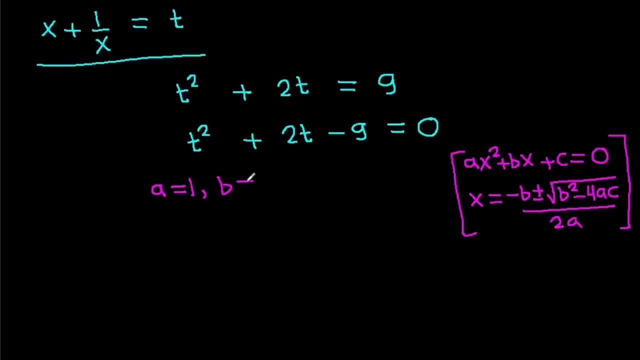 and here a is 1, b is 2 and c is minus 9.. So t it will be minus 2 plus minus s square root of 2s square minus 4 times 1 times minus 9, by 2 times a is 1 and t is equal to minus. 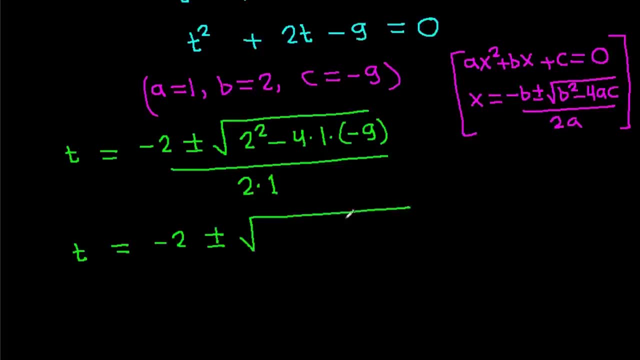 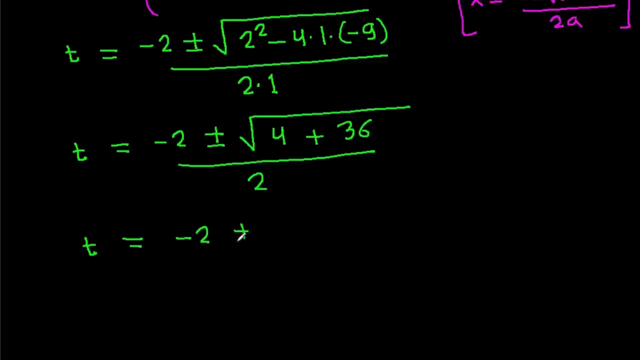 2 plus minus s square root of 4 plus 36 by 2, and t is equal to minus 2 plus minus s square root of 40 by 2, and t is equal to minus 2 plus minus and s square root of 40. it is 2 times s square root of 10 by 2. 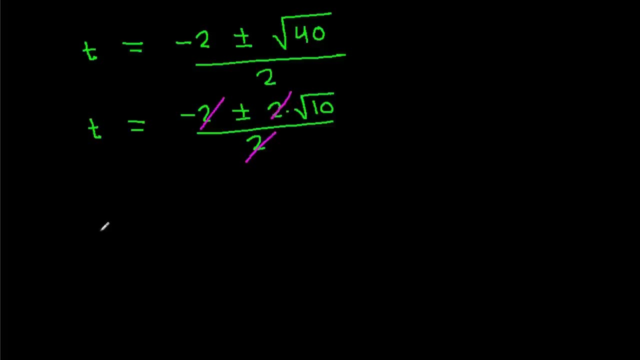 and 2 will get cancelled. so t, it is minus 1 plus minus s square root of 10, and t is x plus 1 by x, that is minus 1, a square root of 10.. So we get x plus 1 by x is minus 1 plus a square root of 10. 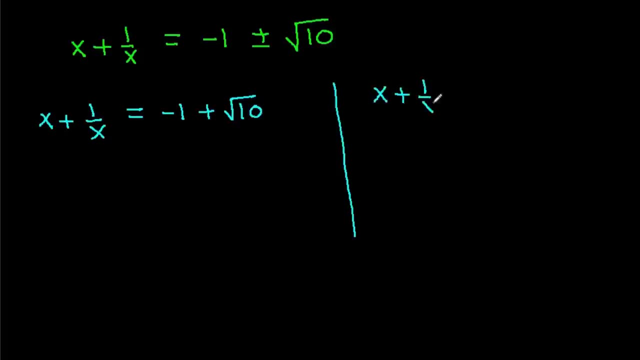 and x plus 1 by x. it is minus 1, minus a square root of 10, and x is length. that should be positive. That means x plus 1 by x. it will be positive and this is negative. So it is not possible. that means x plus 1 by x. it will be a square root of 10. 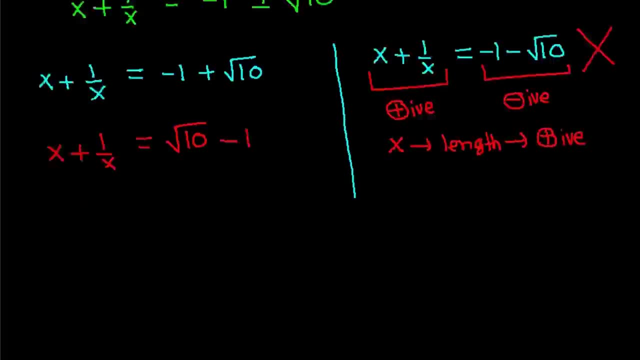 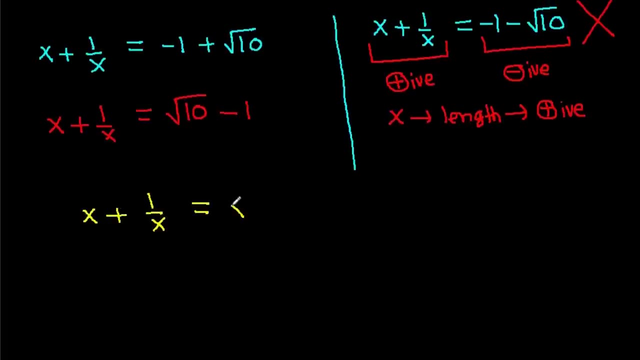 minus 1 and we have x plus 1 by x is a square root of 10 minus 1 and it is x square plus 1 by x is equal to s-square root of 10 minus 1, and if we cross multiply then xs-square plus 1. 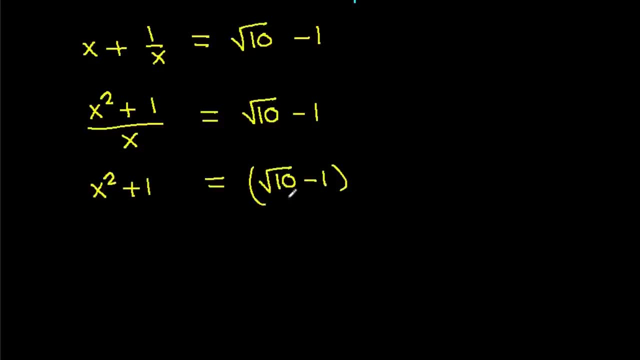 it will be s-square root of 10 minus 1 times x and xs-square minus s-square root of 10 minus 1. x plus 1, it will be equal to 0. and again for equation, axs-square minus bx minus c is equal to 0. x is minus b minus minus s-square root of b-square minus 4ac by 2a. 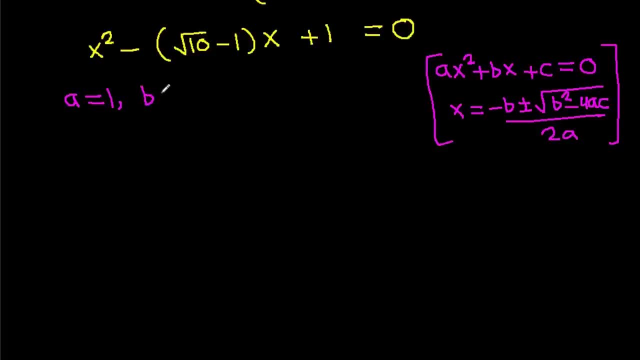 and here we are kupa's equation. that is equal to 0. x minus b minus c minus bx, c is equal. here a is 1, b is minus s square root of 10 minus 1 and c is 1.. So x will be equal to minus of minus s square root of 10 minus 1 plus minus s square root. 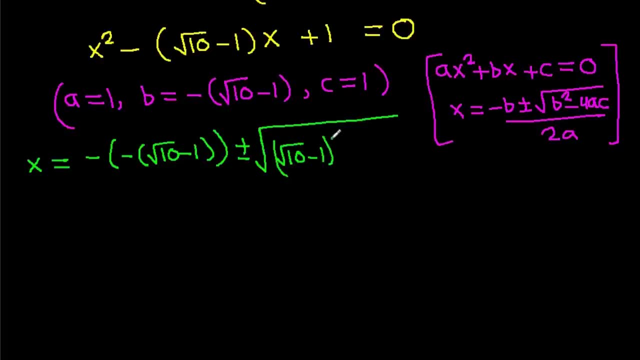 of s square root of 10 minus 1 s square minus 4 times 1, times 1. by 2 times 1 and x is equal to minus times minus will be plus, so it is s square root of 10 minus 1, plus minus s square. 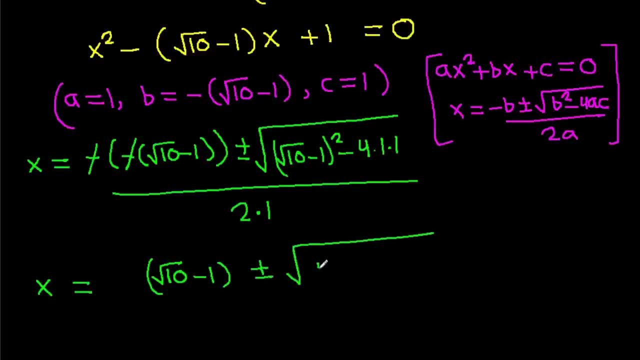 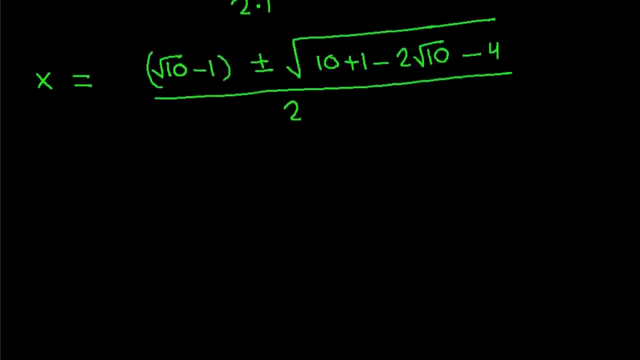 root, And x will be 10 plus 1 minus 2 times s square root of 10 minus 4 by 2, and x is equal to s square root of 10 minus 1 plus minus s square root, and 10 plus 1 minus 4 by 2 times s square. 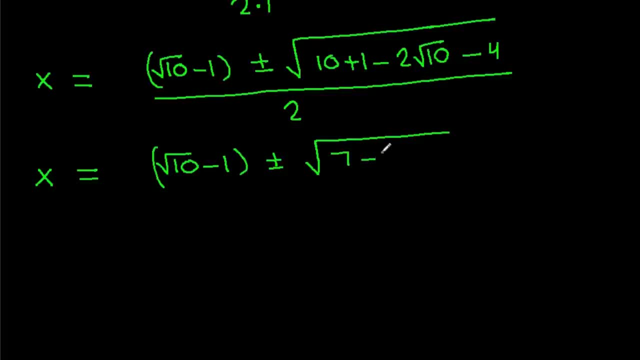 root of 10 minus 1.. it is 7 minus 2 times s square root of 10 by 2 and 7 minus 2 times s square root of 10. it is 5 plus 2 minus 2 times s square root of 10 and 5 is s square root. 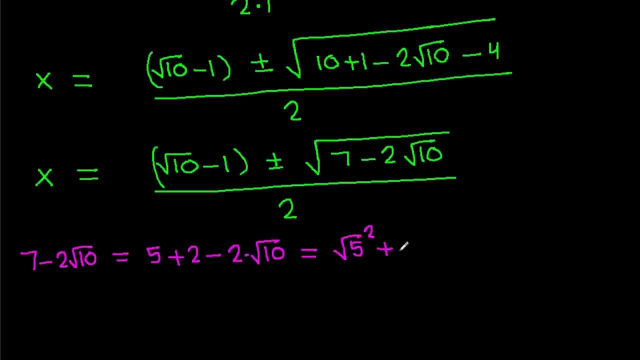 of 5 s square plus 2 is s square root of 2 s square minus 2 times and s square root of 10. it is s square root of 5 times s square root of 2. that will be s square root of 5 minus s square root of 2 s square. 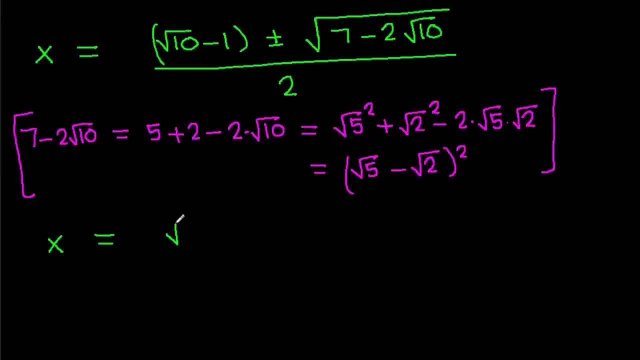 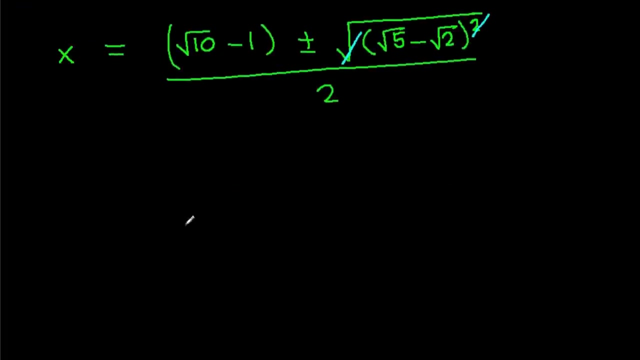 so x is equal to s square root of 10 minus 1 minus minus s square root, and this is s square root of 5 minus s square root of 2, s square by 2 and s square and s square root will get cancelled, and x is equal to s square root of 10 minus 1 plus minus s square root of 5. 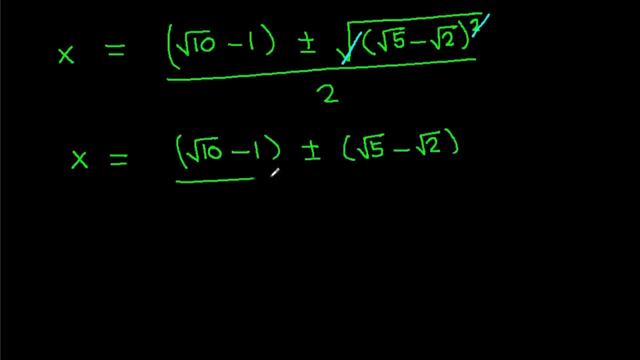 minus s square root of 2 by 2, so we get: x is s square root of 10 minus 1 plus s square root of 5 minus s square root of 2 by 2, and x is equal to s square root of 10 minus 1 minus s square root of 5 minus s square root of 2 by 2, and here it is x. 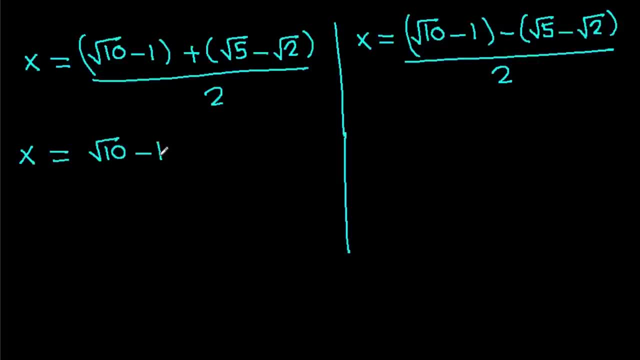 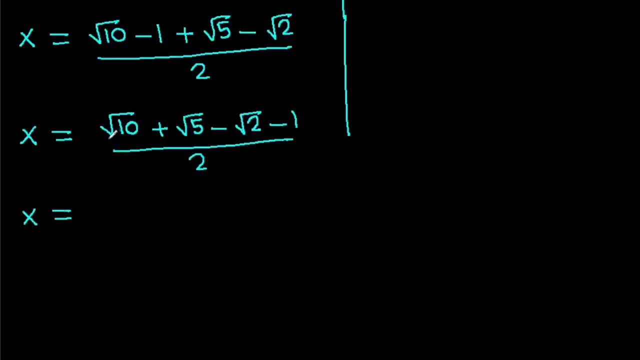 x is equal to s square root of 10. it is s square root of 5 times s square root of 2 minus s square root of 5 minus s square root of 2 minus 1. by 2 and x is equal to: here we can take: 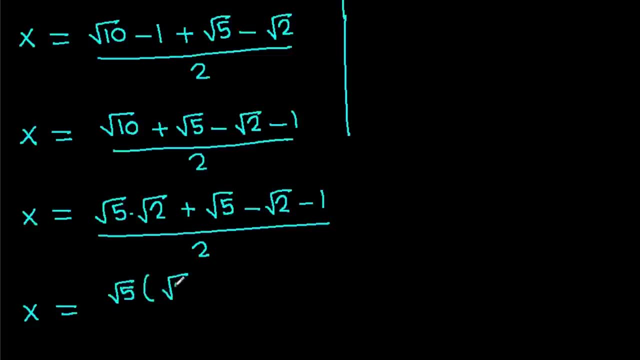 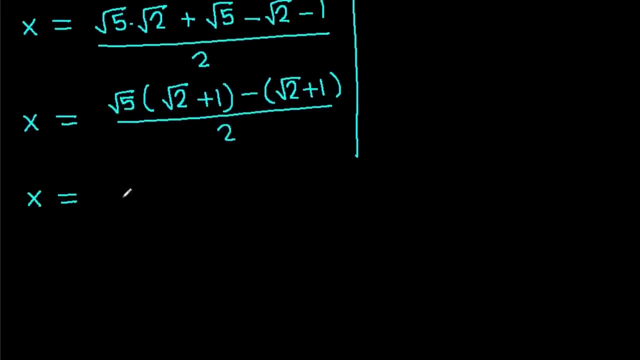 a square root of 5 common, and it will be a square root of 2 minus 1. and here we can take minus common and it will be a square root of 2 minus 1. by 2 and X is equal to, we can take a square root of 2 plus 1 common and it will be a square 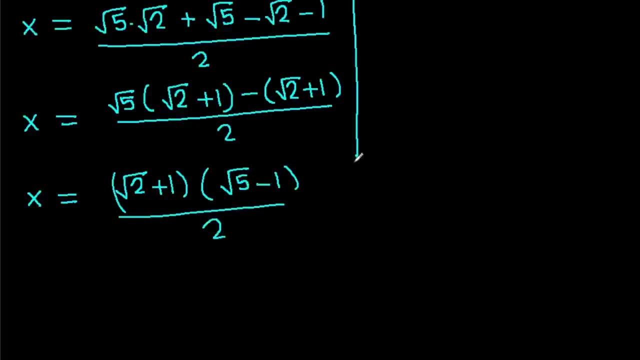 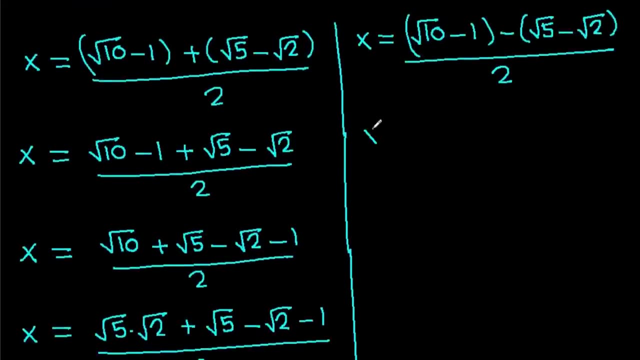 root of 5 minus 1 by 2, and here X is equal to a square root of 10 minus 1, minus a square root of 5 minus a square root of 1.. of 2 by 2 and X is equal to a square root of 10 minus a square root of 5. 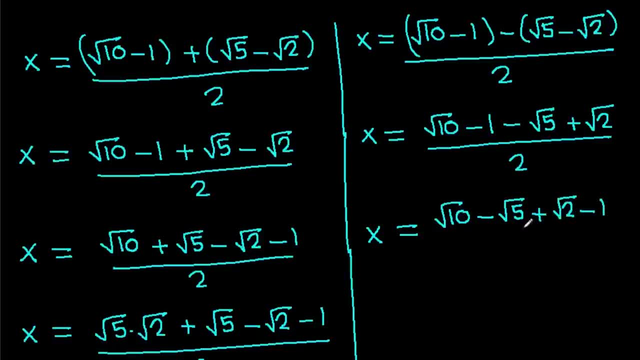 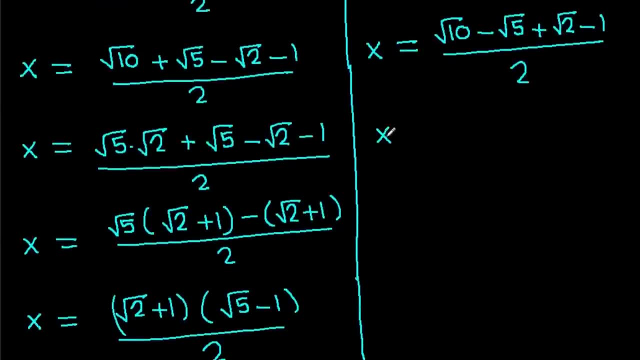 minus a square root of 2 minus 1 by 2 and X is equal to a square root of 10. it is a square root of 5 times a square root of 10.. of 2 minus a square root of 5, minus a square root of 2 minus 1 by 2 and X is: 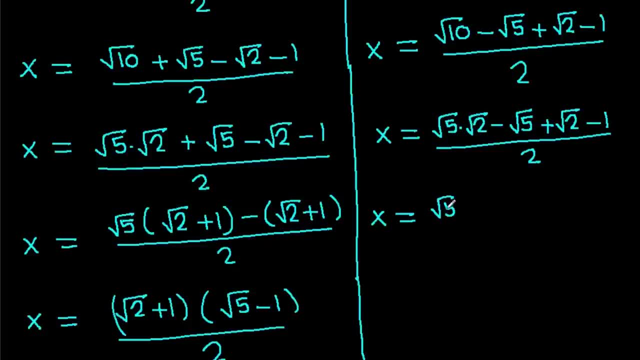 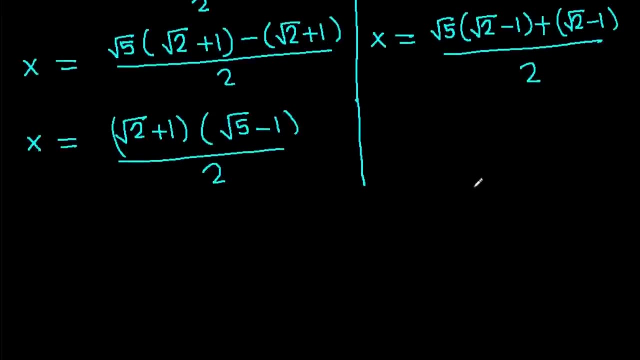 equal to. here: we can take a square root of 5 common, and it will be a square root of 2 minus 1, plus a square root of 2 minus 1 by 2.. and it is X is equal to: we can take a square root of 2 minus 1 common, and it will be a square. 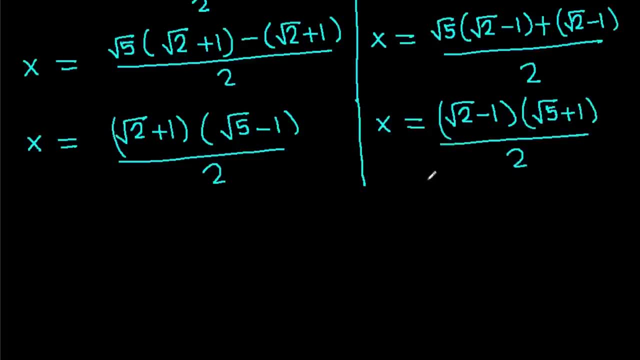 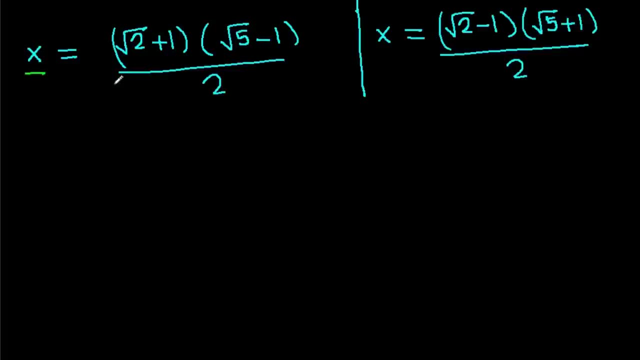 root of 5 minus 1 by 2, and if we multiply these two values of X, then a square root of 2 minus 1 times a square root of 5 minus one by 2 times a square root of 2 minus 1 times a square root of 5 minus 1 by 2.